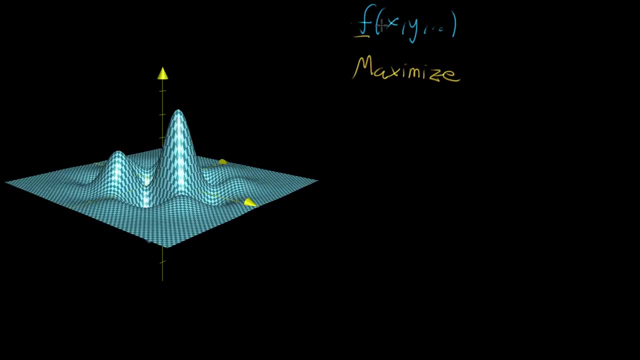 the values of x and y and all of its other inputs, such that the output f is as great as it possibly can be. Now, this actually comes up all the time in practice because usually when you're dealing with a multivariable function, 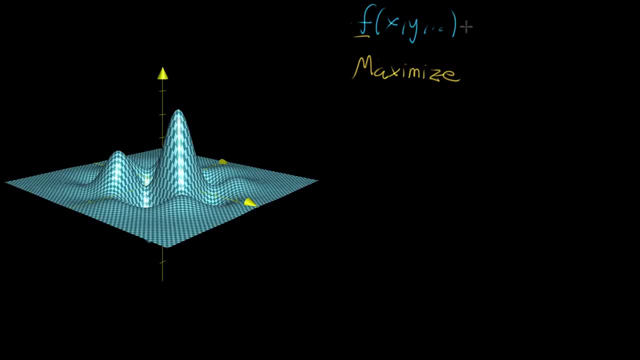 it's not just for fun and for dealing with abstract symbols. it's because it actually represents something. So maybe it represents like profits of a company. maybe this is a function where you're considering all the choices you can make, like the wages you give your employees. 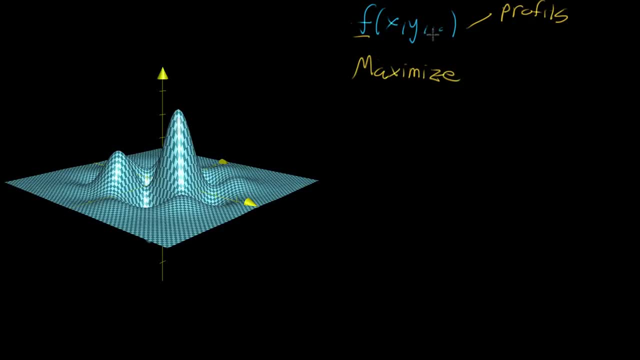 or the prices of your goods, or the amount of debt that you raise for capital, all sorts of choices that you might make, and you wanna know what values should you give to those choices, such that you maximize profits? you maximize a thing, And if you have a function that models these relationships, 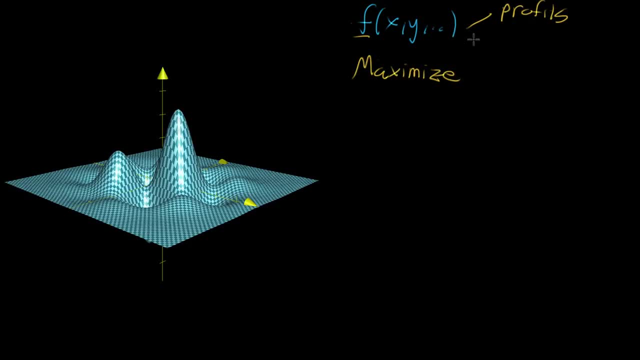 there are techniques, which I'm about to teach you, that you can use to maximize this. Another very common setting, more and more important these days, is that of machine learning and artificial intelligence, where often what you do is you assign something. 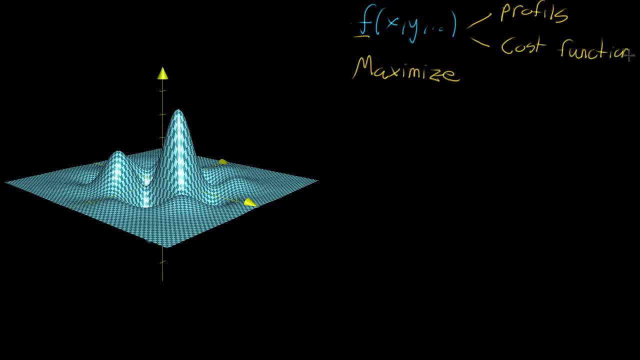 called a cost function to a task. So maybe you're trying to teach a computer how to understand audio or how to read handwritten text. What you do is you find a function that basically tells it how wrong it is when it makes a guess. 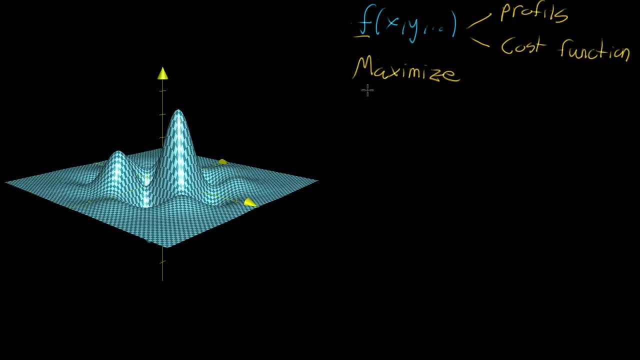 And if you do a good job designing that function, you just need to tell the computer to minimize. so that's kind of the flip side, right: instead of finding the maximum to minimize a certain function, And if it minimizes, this cost function. 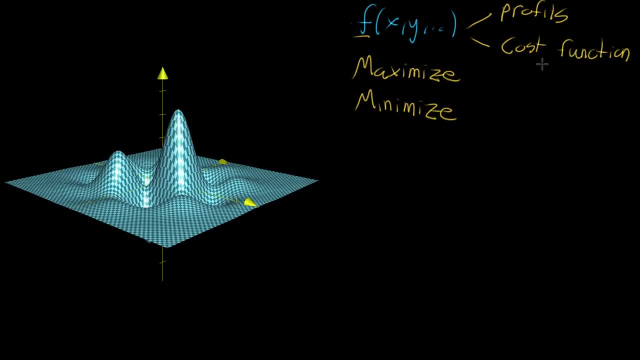 that means that it's doing a really good job at whatever task you've assigned it. So a lot of the art and science of machine learning and artificial intelligence comes down to well one: finding this cost function and actually describing difficult tasks in terms of a function. 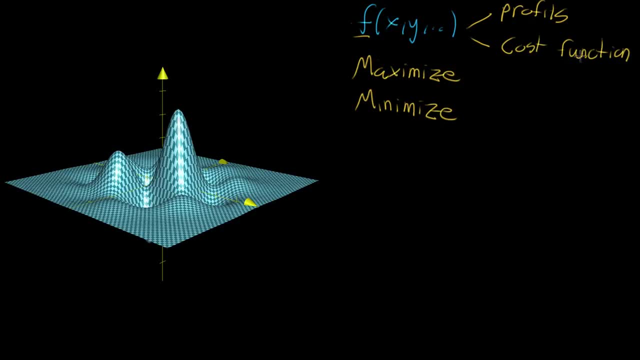 but then applying the techniques that I'm about to teach you, to have the computer minimize that, And a lot of time and research has gone into figuring out ways to basically apply these techniques, but really quickly and efficiently. So first of all, on a conceptual level, 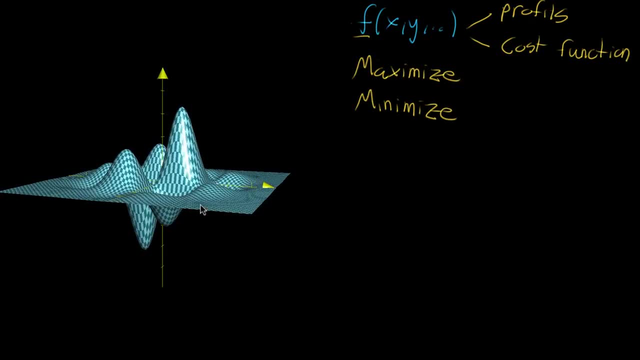 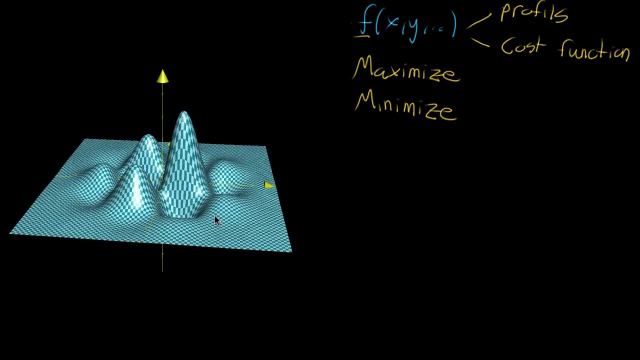 let's just think about what it means to be finding the maximum of a multivariable function. So I have here the graph of a two-variable function. that's something that has a two-variable input that we're thinking of as the xy-plane. 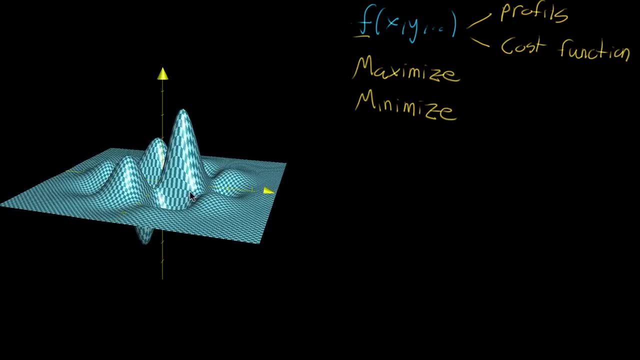 and then its output is the height of this graph And if you're looking to maximize it, basically what you're finding is this peak, kind of the tallest mountain in the entire area, And you're looking for the input value, the point on the xy-plane directly below that peak. 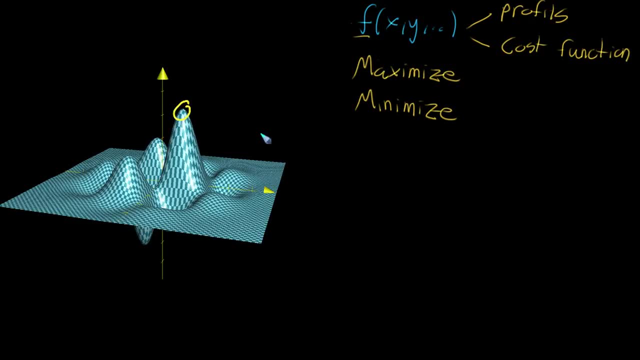 Because that tells you the values of the inputs that you should put in to maximize your function. So how do you go about finding that? Well, this is perhaps the core observation in well calculus, not just multivariable calculus. this is similar in the single variable world. 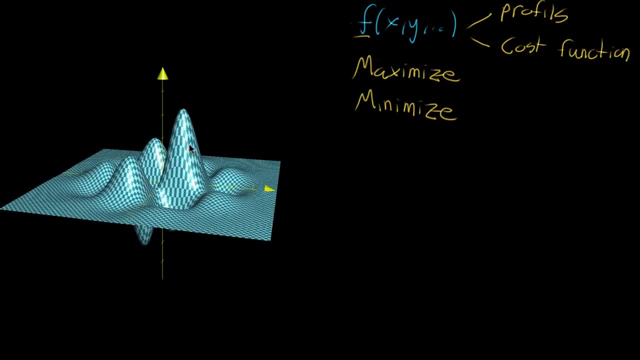 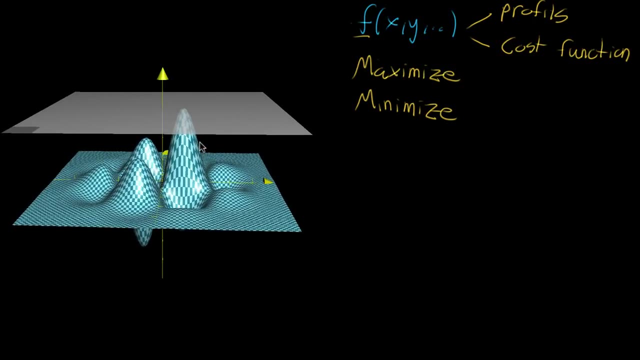 and there's similarities in other settings. but the core observation is that if you take a tangent plane at that peak, so let's just draw in a tangent plane at that peak, it's gonna be completely flat. But let's say you did this at a different point, right? 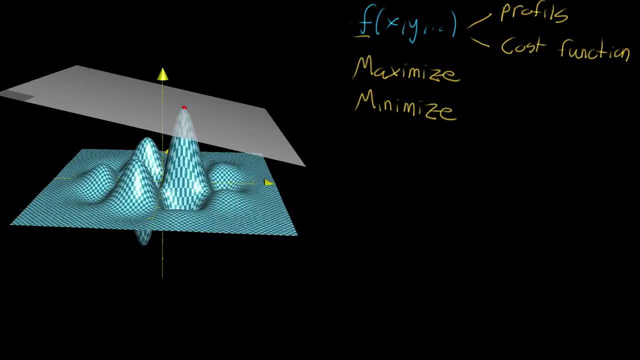 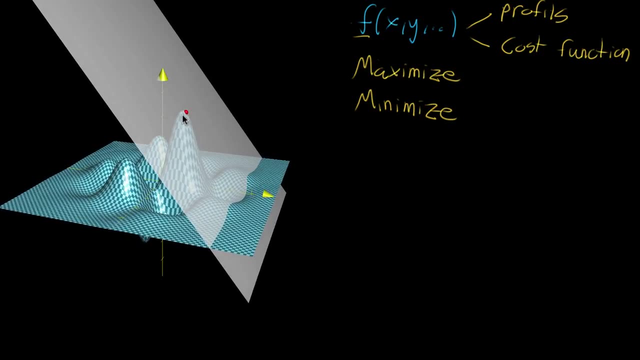 Because if you tried to find the tangent plane- not at that point, but you kind of moved it about a bit to somewhere that's not quite a maximum if the tangent plane has any kind of slope to it- what that's telling you is that if you take 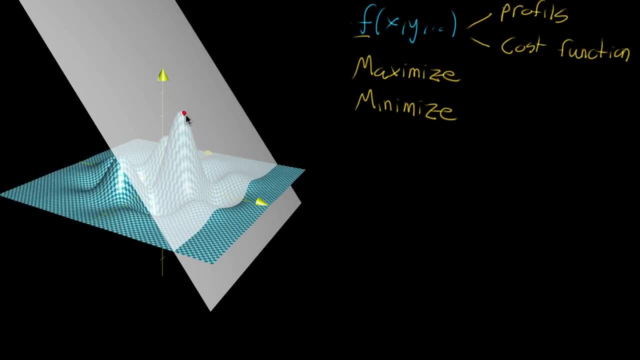 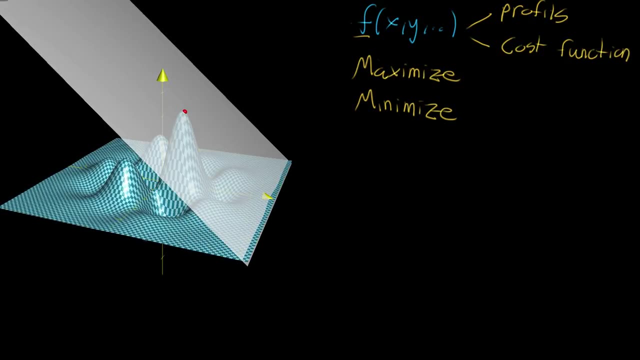 very small directions, kind of in the direction of that upward slope, you can increase the value of your function. So if there's any slope to the tangent plane, you know that you can walk in some direction to increase it. But if there's no slope to it, if it's flat, 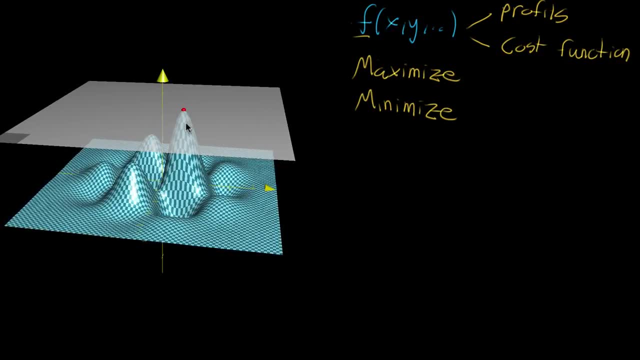 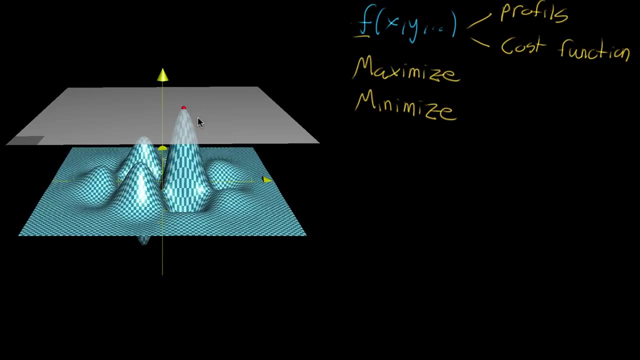 then that's a sign that, no matter which direction you walk, you're not gonna be significantly increasing the value of your function. So what does this mean in terms of formulas? Well, if you kind of think back to how we compute tangent planes, and if you're not very comfortable, 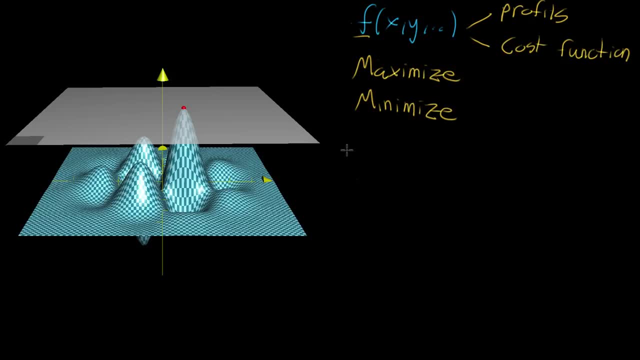 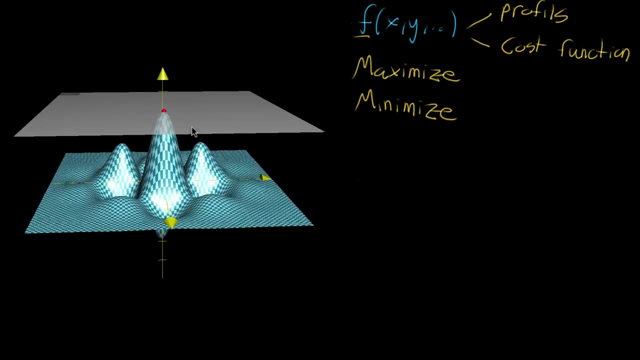 with that. now would be a good time to take another look at those videos about tangent planes, The slope of the plane in each direction. so you know this would be the slope in the x direction and then, if you look at it from another perspective, 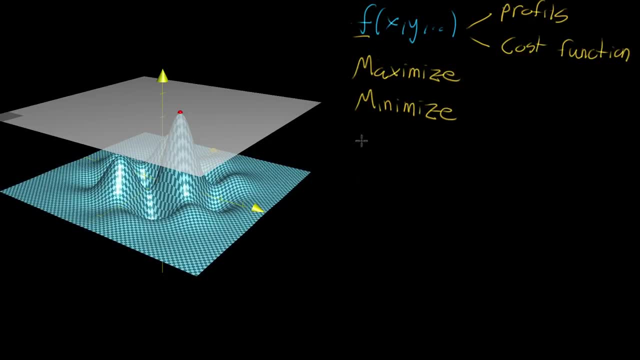 this would be the slope in the y direction. each one of those has to be zero And that, in terms of partial derivatives, means the partial derivative of your function at whatever point you're dealing with, right? So I'll call it x naught, y naught. 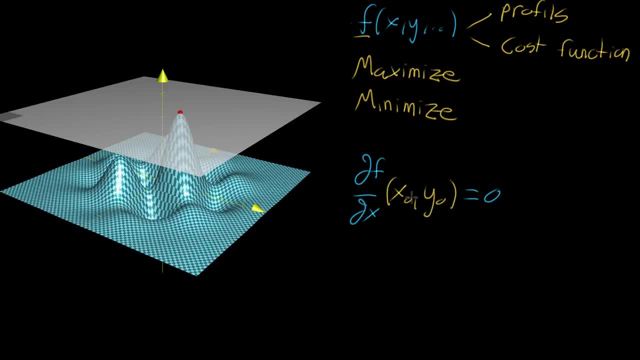 as the point where you're inputting this has to be zero. And then, similarly, the partial derivative with respect to the other variable, with respect to y at that same point, has to be zero, And both of these have to be true. 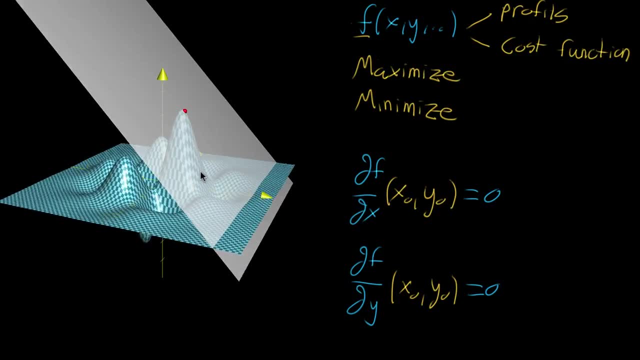 because let's just take a look. I don't know, let's slide it over a little bit here. This tangent plane. if you look at the slope, you imagine walking in the y direction. you're not increasing your value at all. 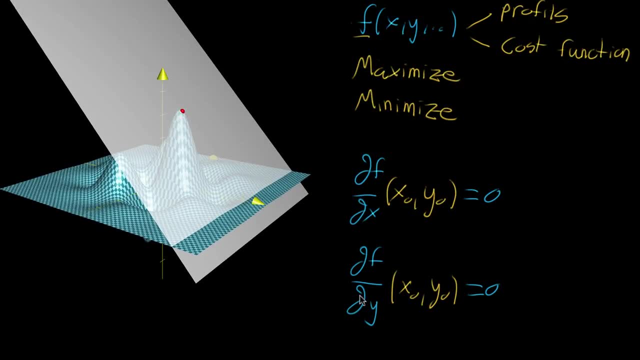 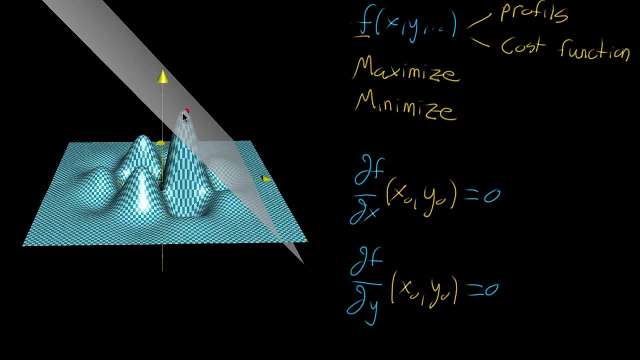 The slope in the y direction would actually be zero. So that would mean the partial derivative with respect to y would be zero. But with respect to x, when you're moving in the x direction, here the slope is clearly negative because as you take positive steps in the x direction, 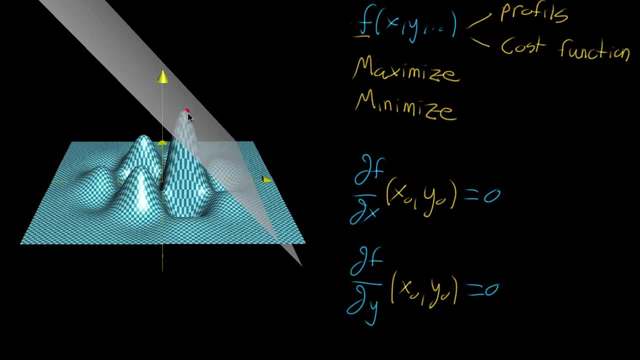 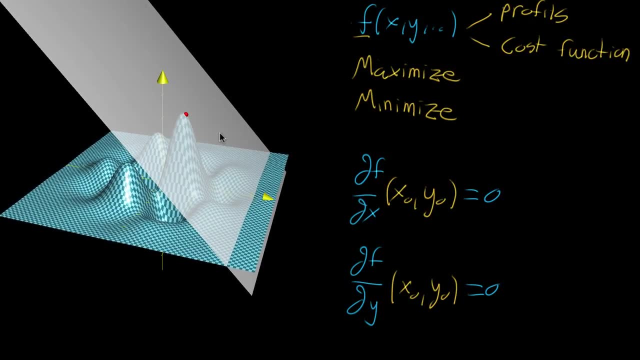 the height of your tangent plane is decreasing, which corresponds to: if you take tiny steps on your graph, then the height will decrease in a manner proportional to the size of those tiny steps. So what this gives you here is gonna be a system of equations where you're solving 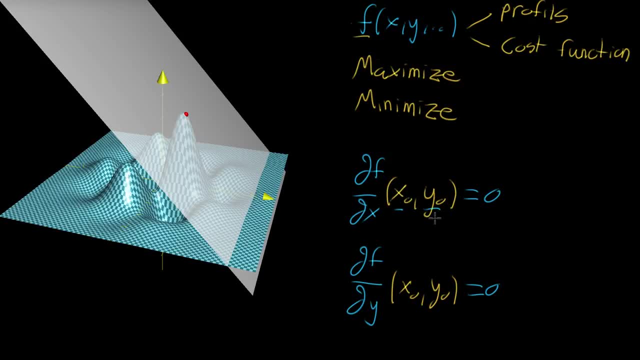 for the value of x naught and y naught. that satisfies both of these equations, And in future videos I'll go through specific examples of this. For now I just want to give a good conceptual understanding. But one very important thing to notice is that 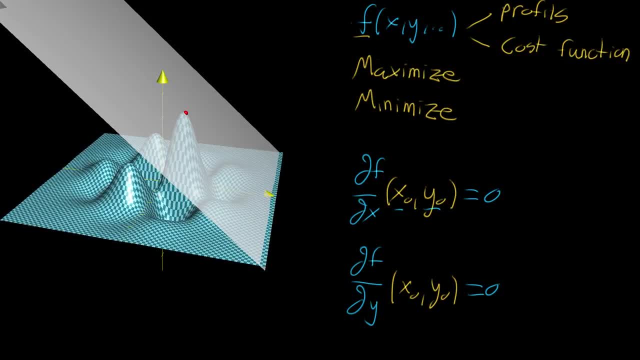 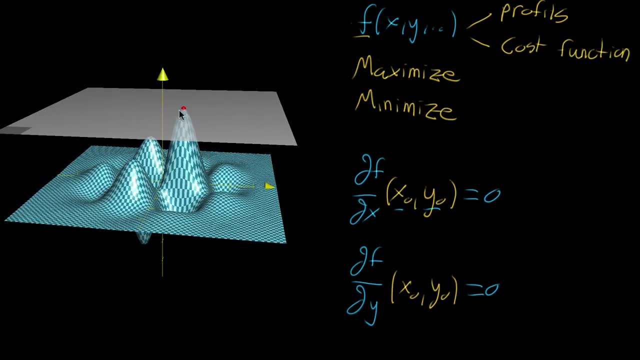 just because this condition is satisfied- meaning your tangent plane is flat- just because that's satisfied doesn't necessarily mean that you've found the maximum. That's just one requirement that it has to satisfy. But for one thing, if you found the tangent plane, 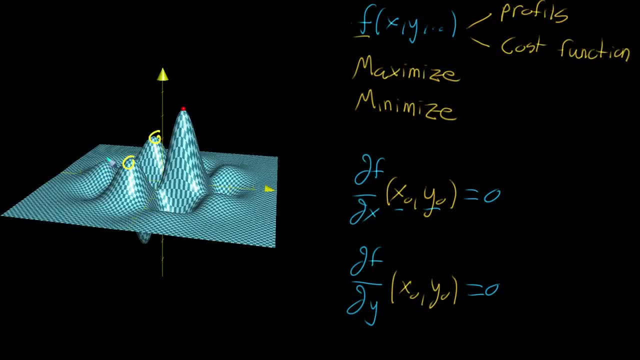 at other little peaks, like this guy here or this guy here or all of the little bumps that go up those tangent planes would also be flat. And those little bumps actually have a name, Because this comes up a lot. they're called. 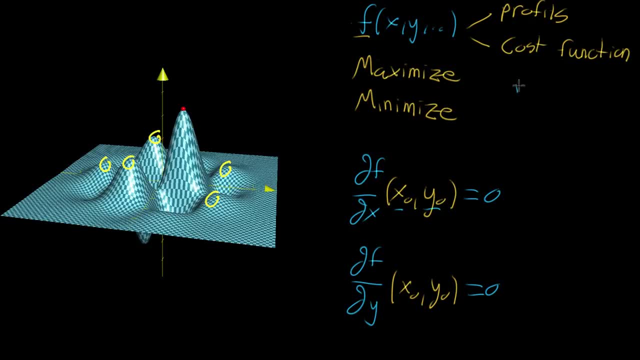 they're called local minima or local maxima. sorry, So those guys are called local maxima. Maxima is just the plural of maximum, And local means that it's relative to a single point. So it's basically if you walk in any direction. 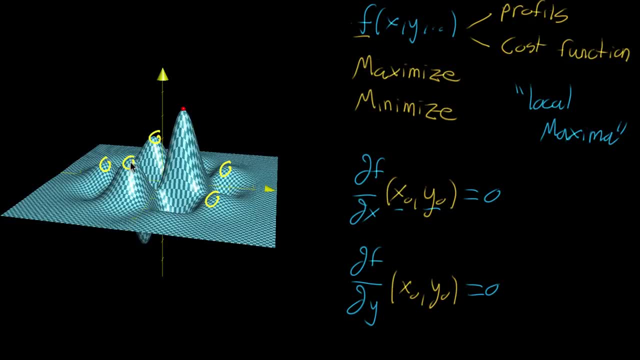 when you're on that little peak you'll go downhill. So relative to the neighbors of that little point it is a maximum, But relative to the entire function. you know these guys are the shorter mountains next to Mount Everest. But there's also another circumstance where you might find. 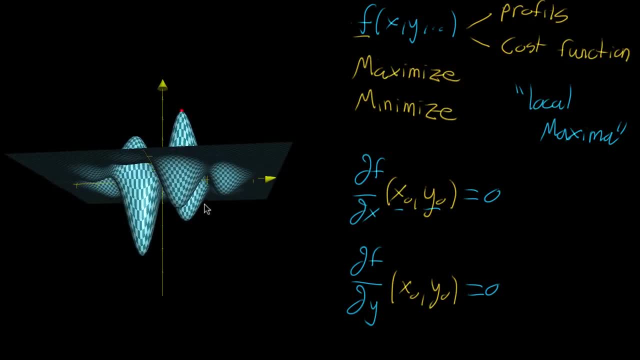 But there's also another circumstance where you might find- But there's also another circumstance where you might find- a flat, tangent plane, And that's at the minima points, right, If you have the global minimum, the absolute smallest, or also just the local minima, these inverted peaks. 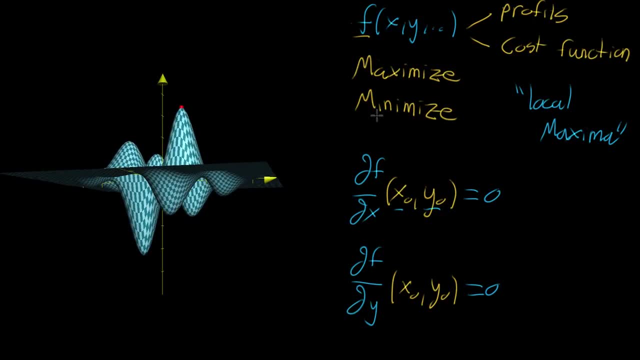 you'll also find flat tangent planes. So what that means first of all is that when you're minimizing a function, you also have to look for this requirement, where all the partial derivatives are zero, But it mainly just means that your job isn't done. 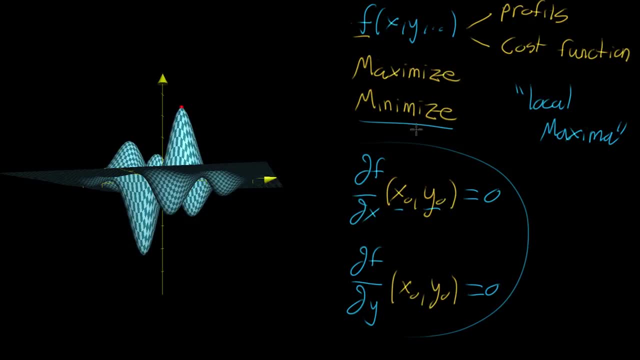 once you've done this, You have to do more tests to check whether or not what you found is a local maximum, or a local minimum or a global maximum. And these requirements, by the way, often you'll see them written in a more succinct form. 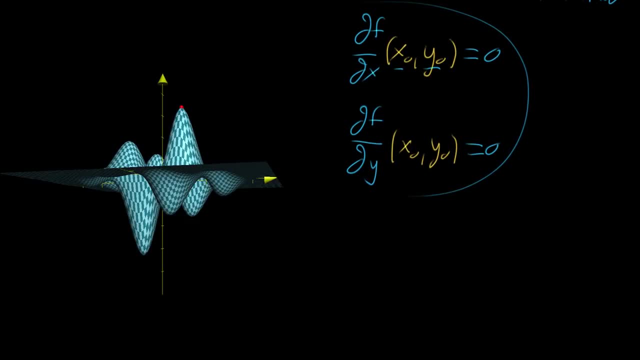 where, instead of saying all the partial derivatives have to be zero, which is what you need to find- they'll write it in a different form, where you say that the gradient of your function f, which of course is just the vector that contains all those partial derivatives.